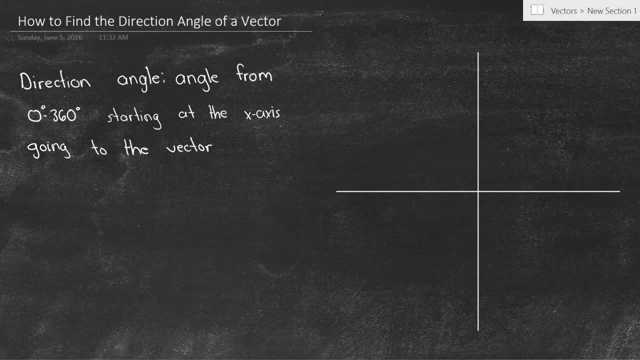 starting at the x-axis and going to the vector. I know this can be confusing, so I'm going to draw some pictures and we'll figure out what direction angles are. So let's say, we have here and we have, well, what's our direction angle of this going to be? 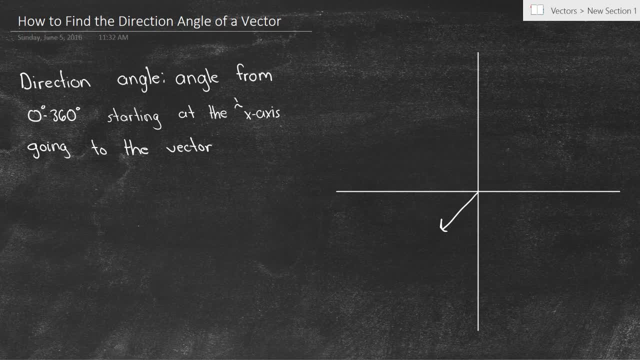 We're going to start at the x-axis. I should say positive, x-axis, positive. you can also think of it as the start of the unit circle, If you've gotten that far. I just wanted to make sure anyone could understand. So we're starting at the positive x-axis and we're going all the way to this vector. 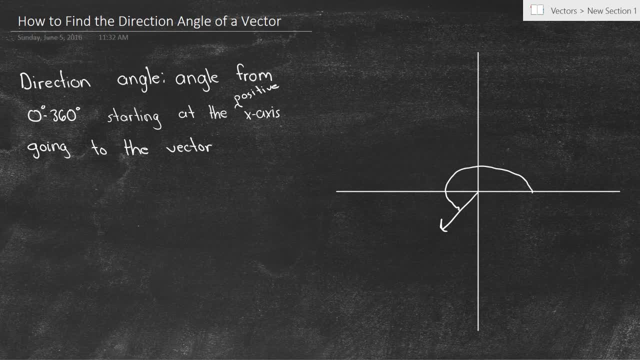 So we're going from there all the way to there And that would be our unit vector. I mean, that would be our direction angle, not unit vector. So that's that one. and then let's try another point. Let's say we've got here, the direction angle is going to be all the way there. 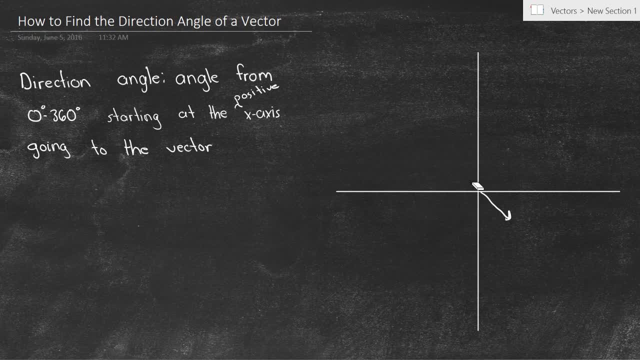 That angle, that degree measure, That degree measurement will be the direction angle. Okay, so now you understand what the direction angle is, and now let's figure out the hard part, which is how to calculate it. So let's start with a pretty simple example. 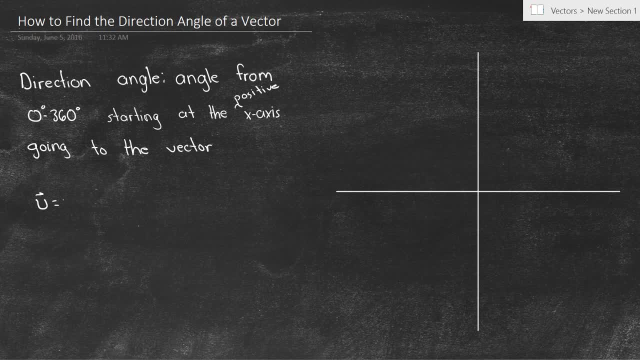 Let's say we've got the vector, we'll call it u and it's going to equal. we'll say 4, 4.. So we've got 1, 2, 3, 4, 1,, 2,, 3, 4.. 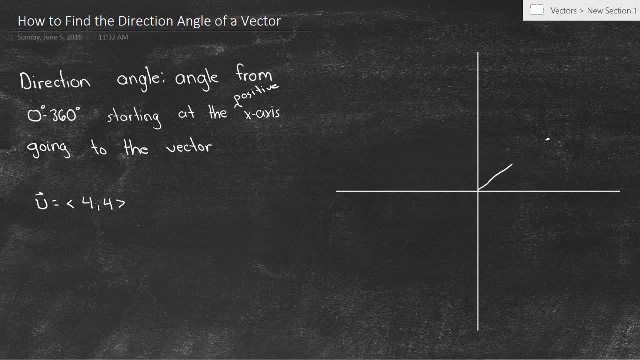 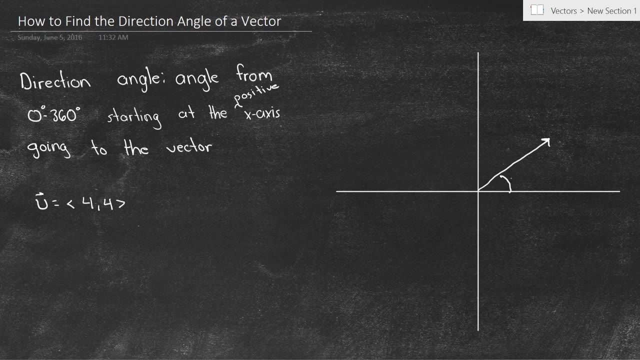 We've got it like here or something, and that's the terminal point, and we'll start it at the origin, just so it'll be easy for us. and now let's think: well, what's the direction angle? We're starting at the positive x-axis and going to the angle. we're going to be looking for this angle. 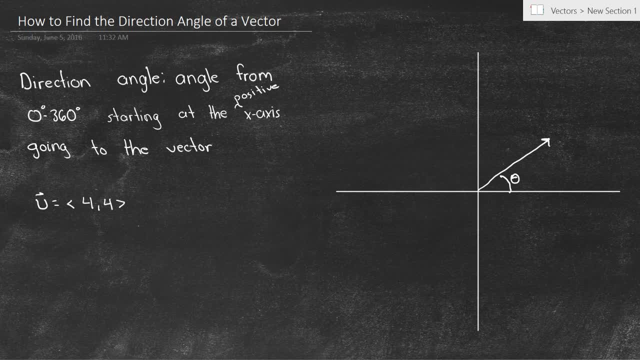 And now we need to think back to our trig. How do we figure out the theta measurement for something like this if we know that this is 4, and we also know that this is 4?? Well, what we know is: we know the opposite and the adjacent. 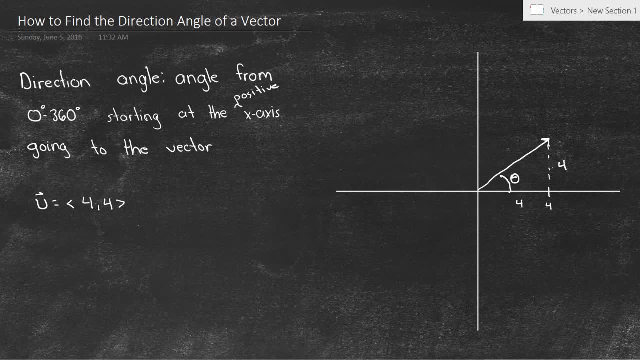 So we know this is 4, and that's 4, so we know that, well, tangent inverse of theta equals opposite over adjacent. so it's going to equal 4 over 4, so then I, well, tangent of theta is going to equal 4. 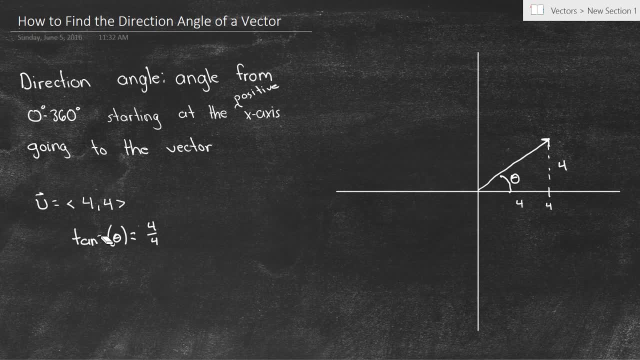 over 4,. I should say tangent of theta, not tangent inverse theta. let me x that out. So: tangent inverse of 4 over 4, you can put this into your calculator. tangent inverse of 1, let's see what you should. 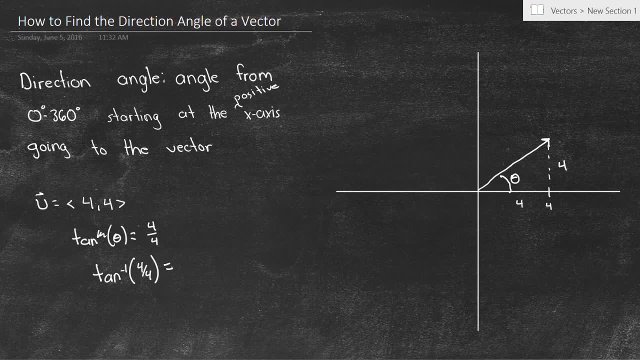 You should get. we just have to think about: well, when is tangent equal to 1, that's going to be 45 degrees. So the direction angle for the vector 4, 4 is 45 degrees. But now we need to get into some harder examples, because this is when it can get confusing. 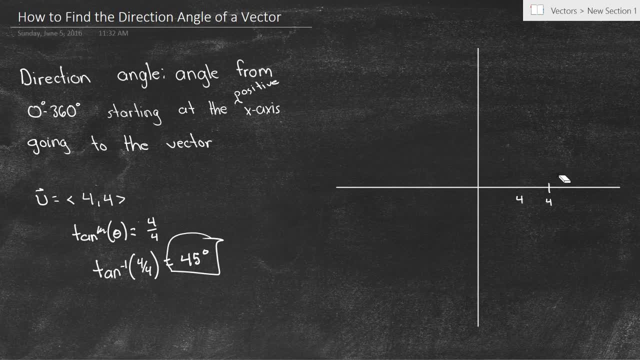 So let's say we're given- let me erase this real quick, So that one's pretty straightforward- You just solve it immediately and you get your angle and you don't have to add anything or subtract anything. But then let's say we had this: 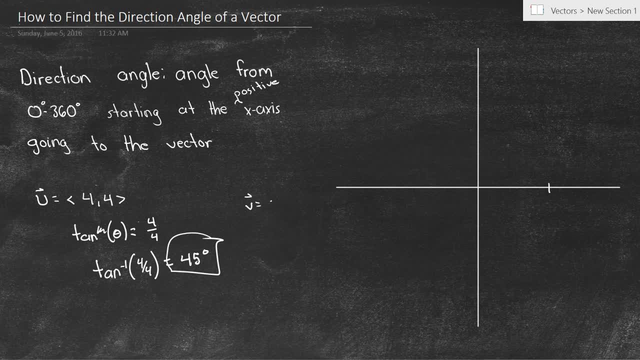 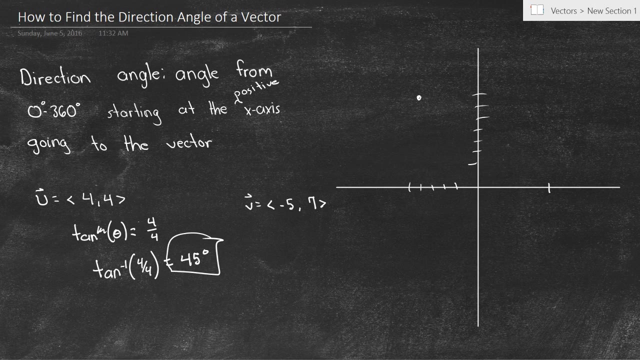 Let's say we had this vector, we'll call it v, and it's at the point negative 5, 7.. So negative 5, 1,, 2, 3, 4, 5, 1, 2,, 3, 4, 5,, 6, 7, we're somewhere up here and it's. 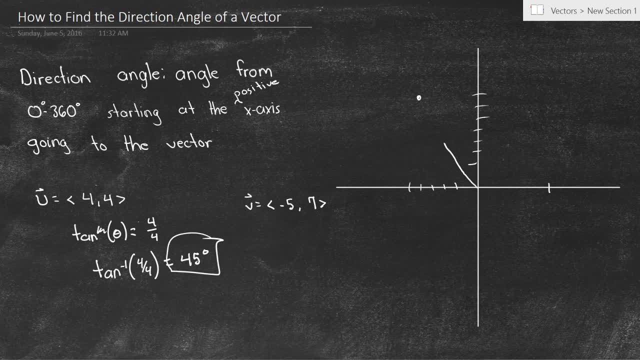 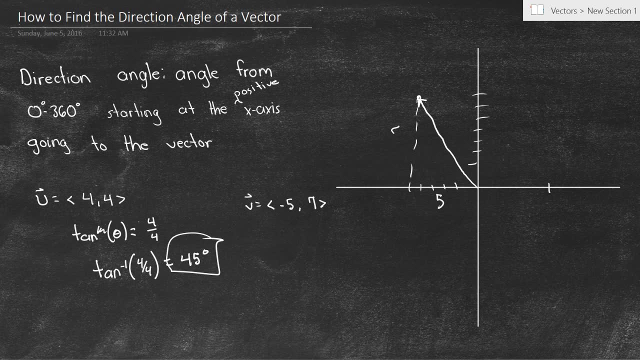 going, starting at the origin. so we're going up like this: we know this is 5,, we know this is 7.. So again, we're going to be using this vector. we'll call it v and it's at the point, negative. 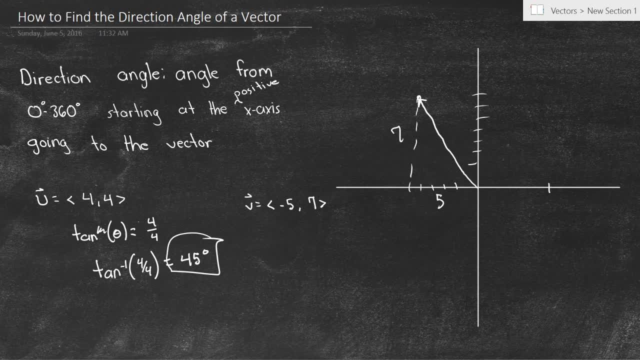 5, 7.. So, again, we're going to be using tangent. but let's think about it. The angle that we're the direction angle is this: This I'll say direction angle, But when we solve using our inverse tangent thing, we're going to be getting this angle. 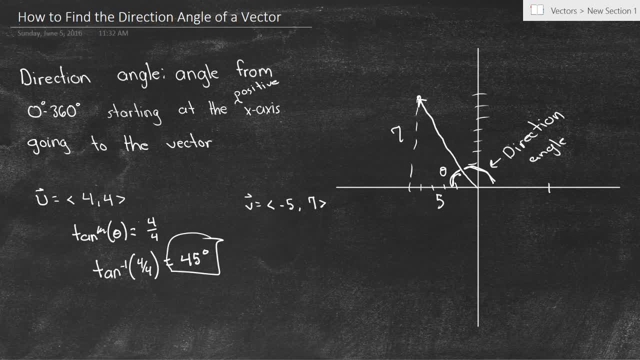 right here. So let's just be careful. So we're going to have tangent of theta equals. again, it's our opposite over our adjacent, which is 7 over 5.. So then to get that by itself, we have to do tangent over 5.. So again we're going to be using this angle right here. So then we're going to have tangent of theta equals. again it's our opposite over our adjacent, which is 7 over 5.. So we're going to have tangent inverse of 7 over 5.. 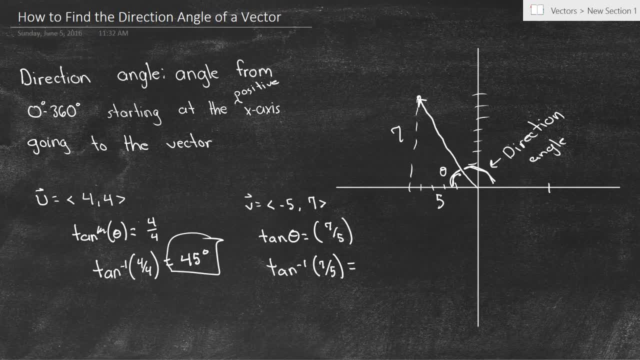 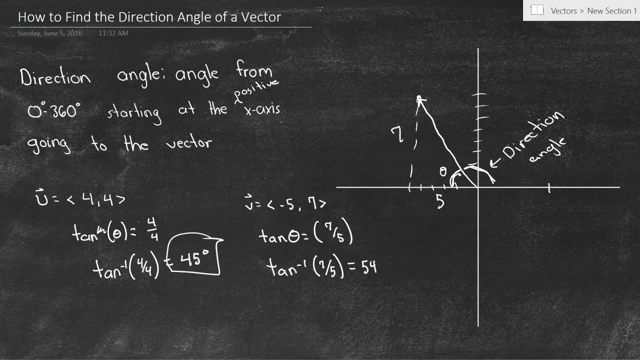 And that's going to equal. let's see, Let me use my calculator here. I don't know that. one by heart, I apologize. 7 divided by 5, we're going to get 54.46 degrees. So 54.46 degrees.